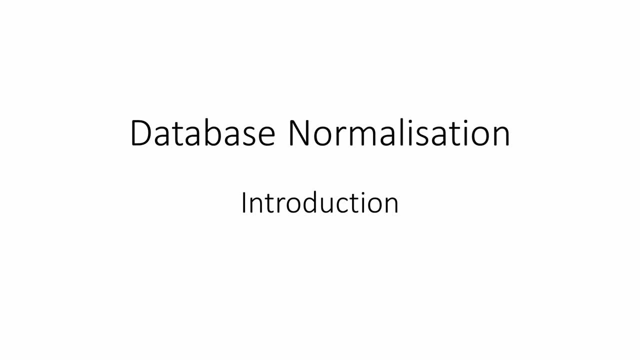 In the videos that follow. I'll explain these definitions in plain English by working through an example that you can understand. So what is database normalization? Once you've decided what data you need to store in a database, at least in general terms, then you need to work out what tables you're going to need. 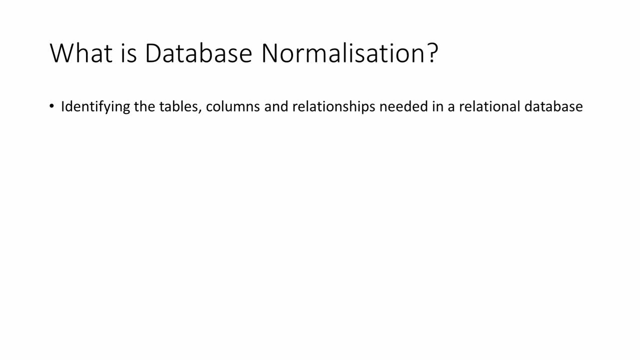 You need to know what columns each table will have and you need to identify the relationships between the tables. Normalization is a formal process that will allow you to do this. It's a well-documented, systematic approach to organization. It's not just organizing the data in a relational database. 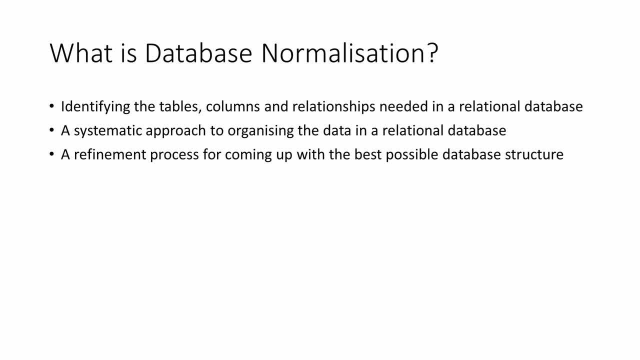 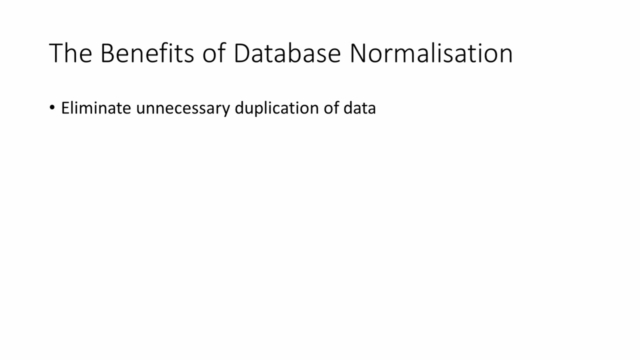 It's a refinement process through which you can derive the most efficient structure for a database. During the normalization process, a relational database is transformed from one normal form to the next until an optimal structure is arrived at. Database normalization rarely eliminates all duplication of data. 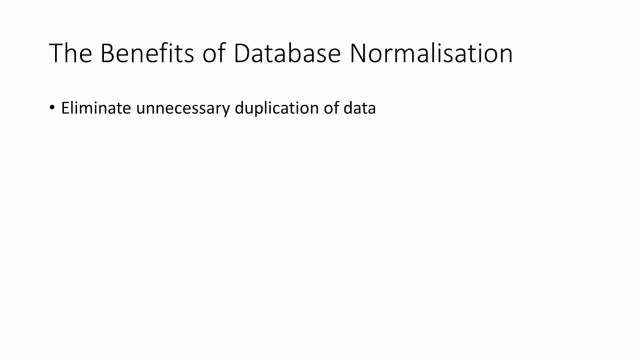 But what it does do is eliminate unnecessary duplication of data. This means that a normalized database is more space efficient. If it's only possible to edit a particular data item in one place, for example somebody's surname, then there's no possibility of having different values for the same thing in different places. 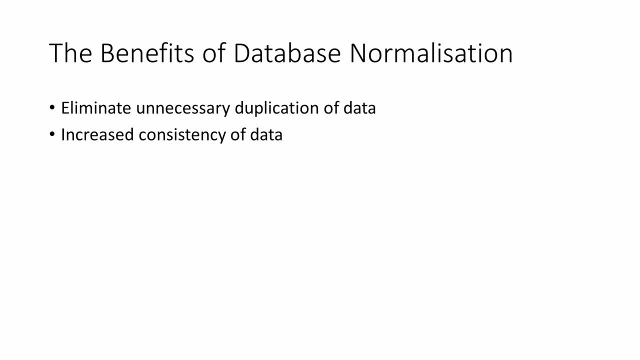 Data are consistent. One of the key features of object-oriented programming is the way that real-world data is stored. It's the way that real-world entities are modeled with classes and the way that multiple objects of the same type can be created from these classes. 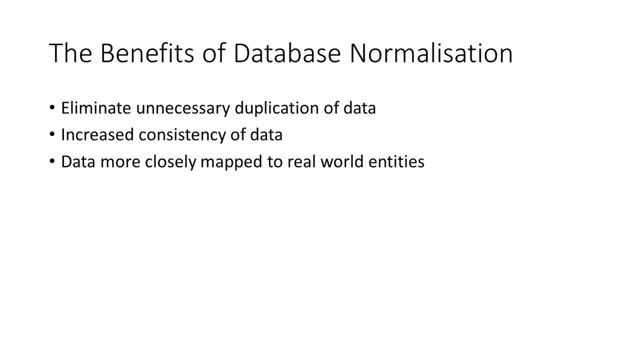 Often, the data contained within a programmatic object is persisted as a record in a database. A normalized relational database lends itself well to this job if it, too, is more closely mapped to real-world entities. If you ever develop an application with a database at the back end. 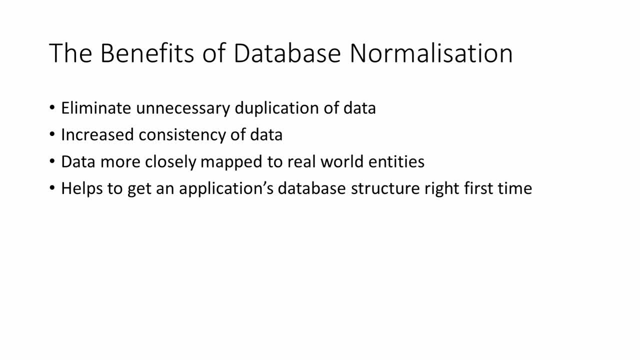 you may experience the frustration of realizing well into the project that the database structure you established in the first place isn't fit for purpose. Normalization is a process that will help you to get it right first time, and this can save you a lot of recoding later.